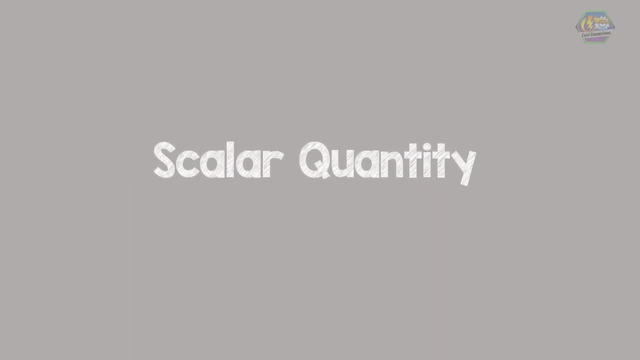 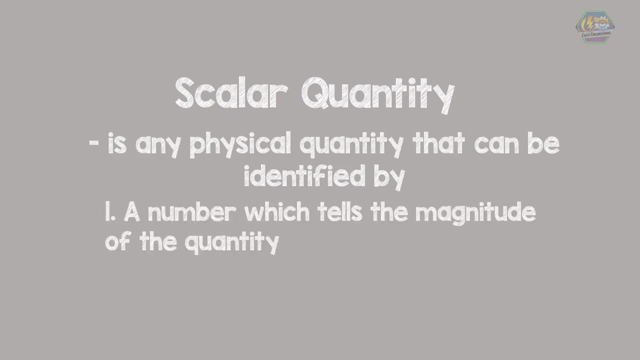 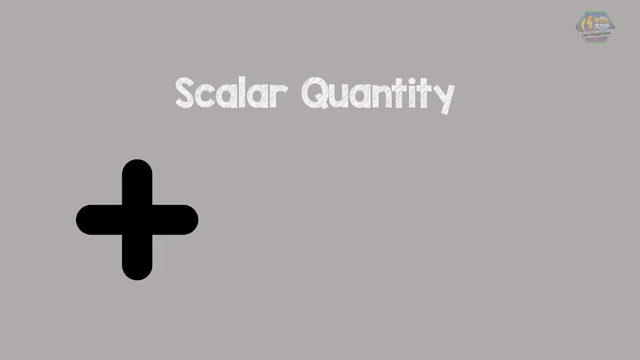 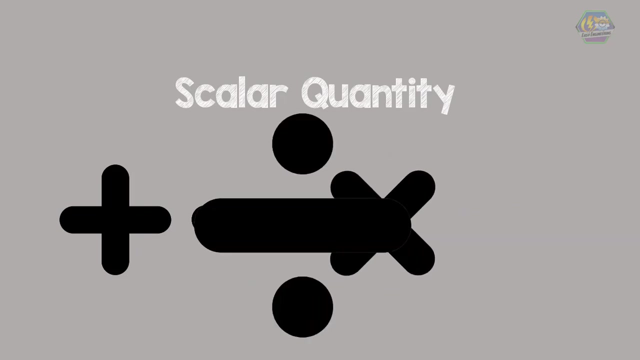 So first let's discuss the scalar quantity. A scalar quantity is any physical quantity that can be identified by number 1, a number which tells us the magnitude of the quantity, number 2, an appropriate unit. Scalar quantities can be added, subtracted, multiplied and divided by common algebraic laws. 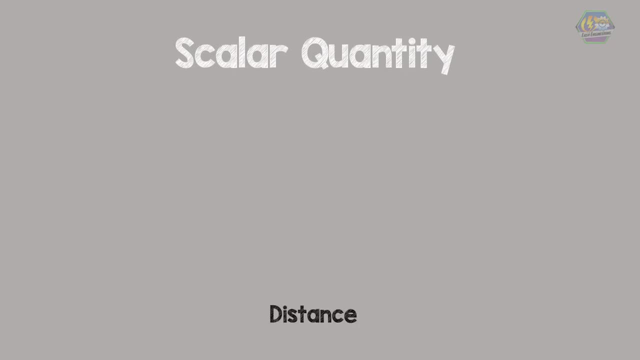 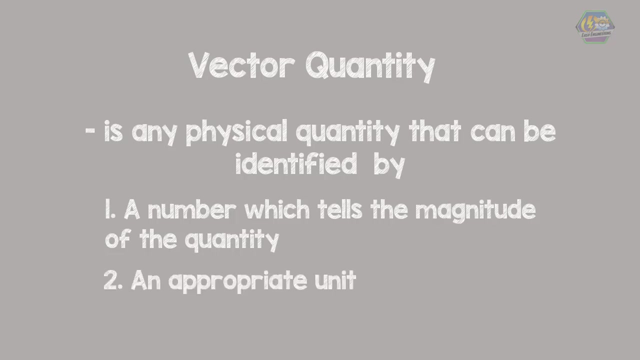 Such examples are distance, mass, temperature, energy and many more. And now, on the other hand, is the vector quantity. A vector quantity is any physical quantity that can be identified by number 1, a number which tells us the magnitude of the quantity, number 2, an appropriate unit, and number 3, a specific direction. 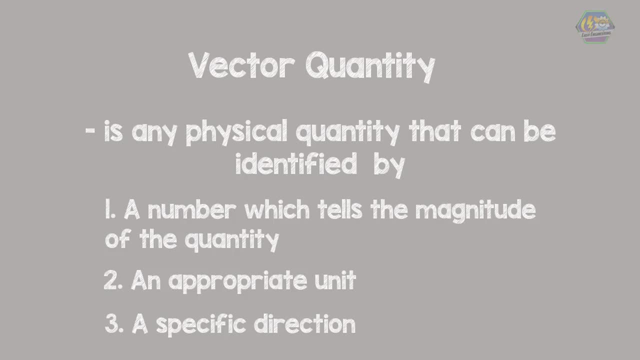 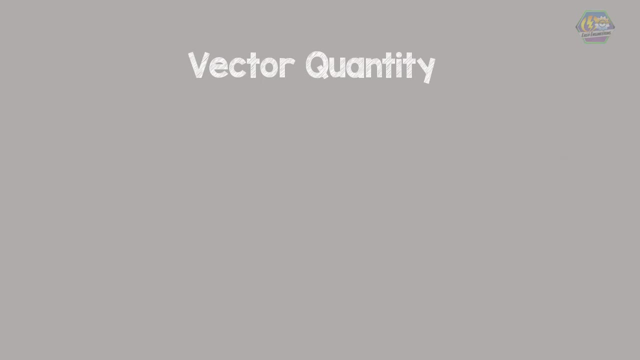 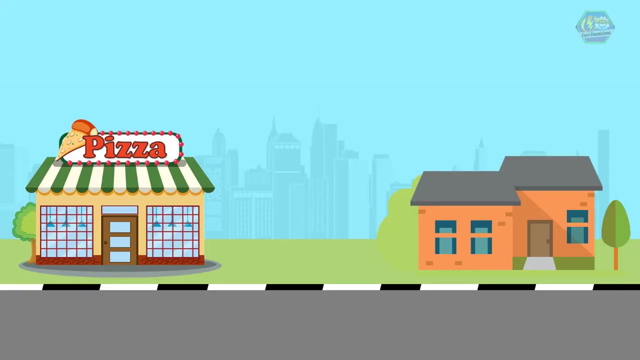 This means that a vector is both a uni-direction and a representation of a quantity and its direction. this includes displacement, velocity, acceleration and many more. For example, imagine yourself calling for a pizza delivery. Then the pizza owner asks you: where do you live? 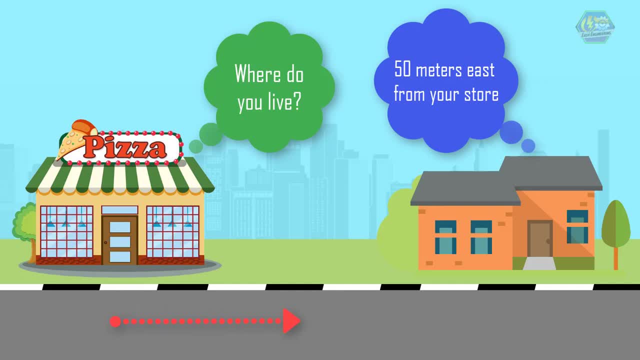 Then you reply 50 meters east from your store. The 50 meters east is a vector quantity because both quantity and direction is present. But when you reply to the pizza gay Islam by text ents to the error. when a line is not terus to be tucked, it will get a force to cook балawin. 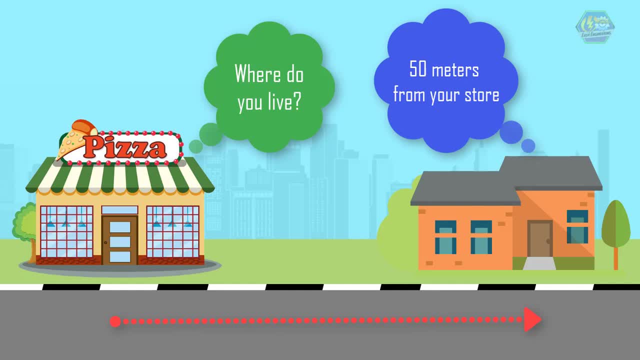 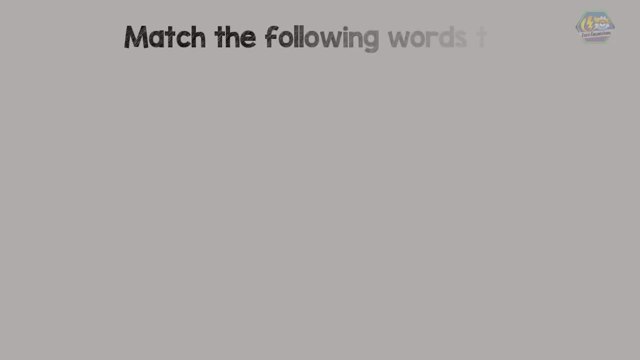 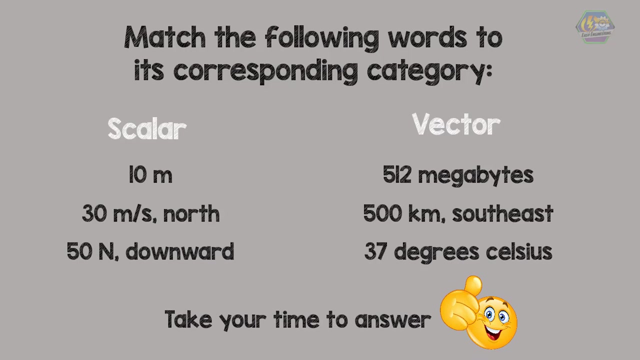 to the pizza owner 50 meters from your store. it will only create confusions because the direction is not specified here. 50 meters is an example of scalar quantity. now let us check your understanding by matching the following words to the corresponding category. let us check your answer. 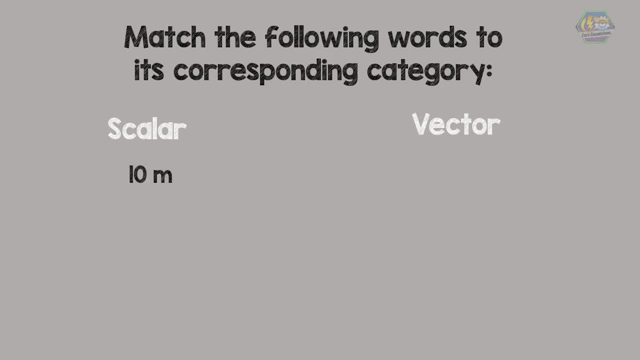 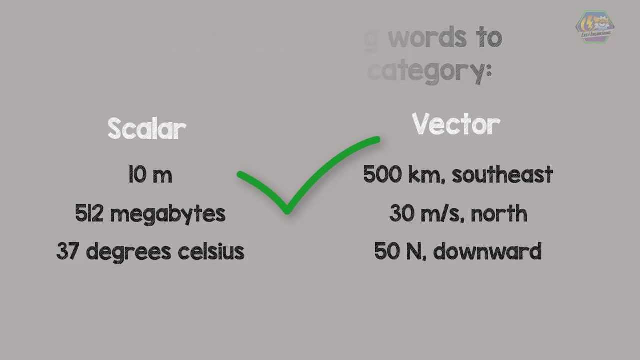 under scalar are 10 meters, 512 megabytes and 37 degrees celsius, and under vector are 500 kilometers southeast, 30 meters per second north, 50 newton downward. i hope you got everything right. that is all for now. i hope you learned something today once again. this is easy engineering. 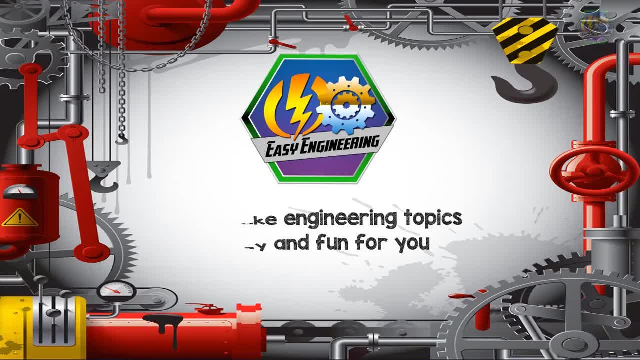 so thank you for watching and i will see you in the next video.